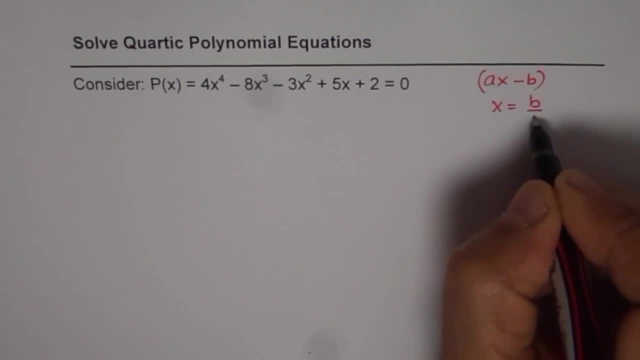 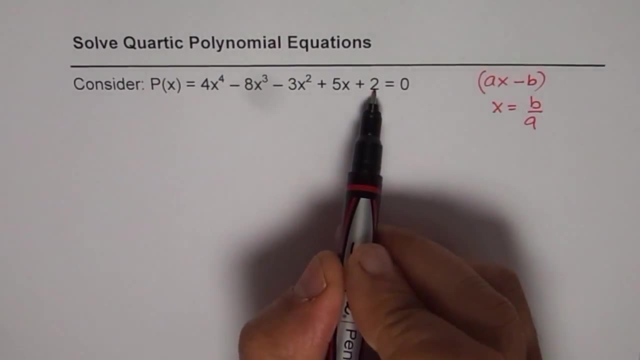 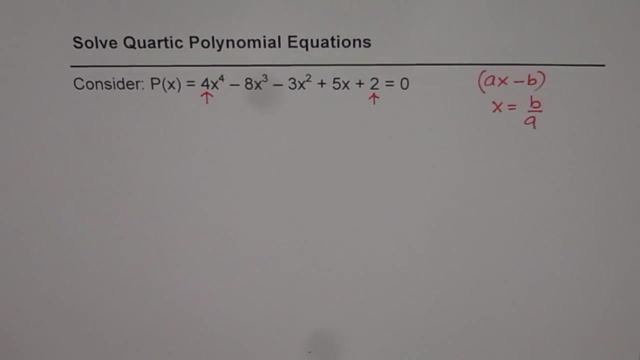 if x is equals to b over a right. So we are trying to find possible values of b over a which we get by the factors of constant and the leading coefficient right. So these are the possible values which can help us find the answer correct. So we should always begin by writing down the possible numbers which could give us a possible values of b over a. 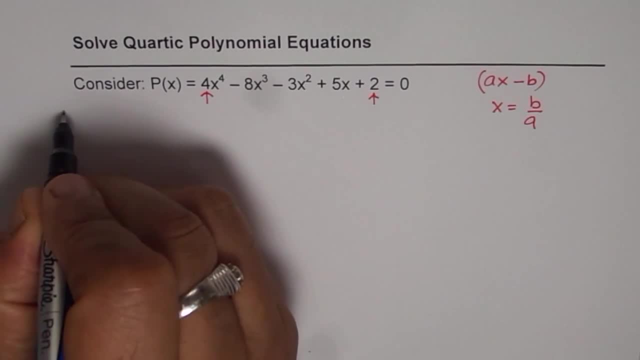 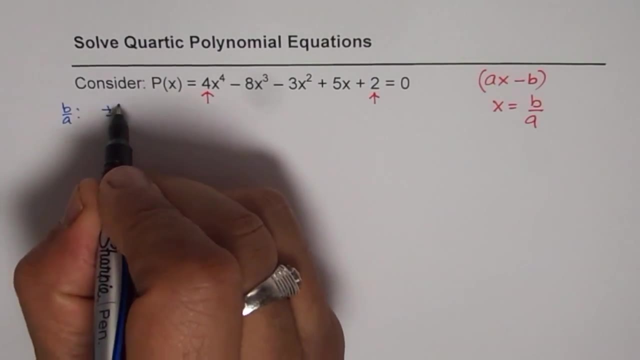 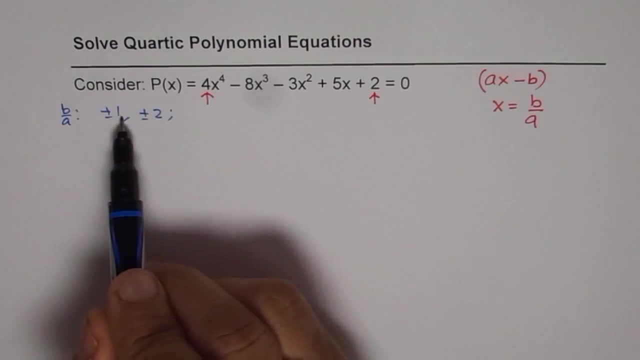 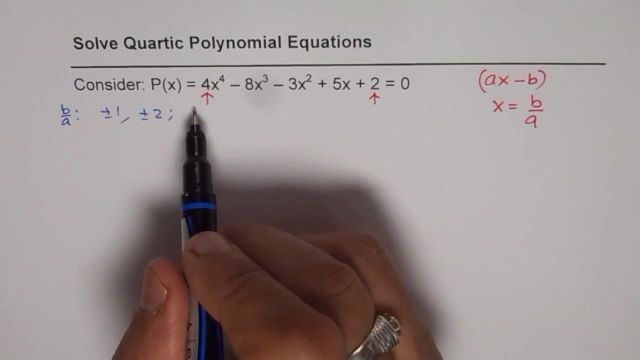 right, which could give us a 0 right. So the possible factors are so we can write. possible values of b over a are first factors of 2, which are plus minus 1 and plus minus 2, and then factors of 2 divided by factors of 4.. Well, when we say this, we have divided them by 1, correct. Now let's divide them by factors, other factors of 4, like 2 and 4.. So when I divide by 2, I get plus minus half. 2 divided by 2 is 1, which is 0. 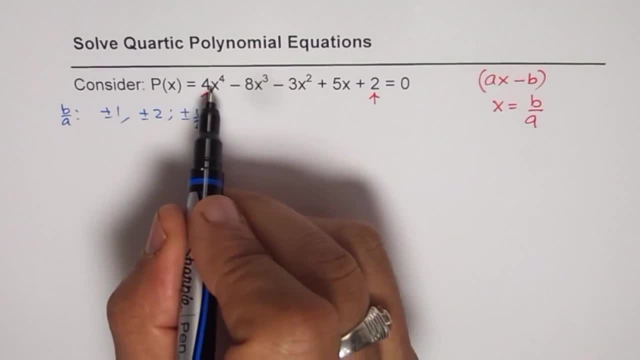 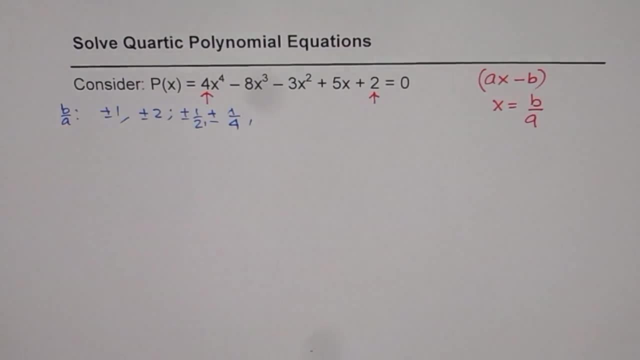 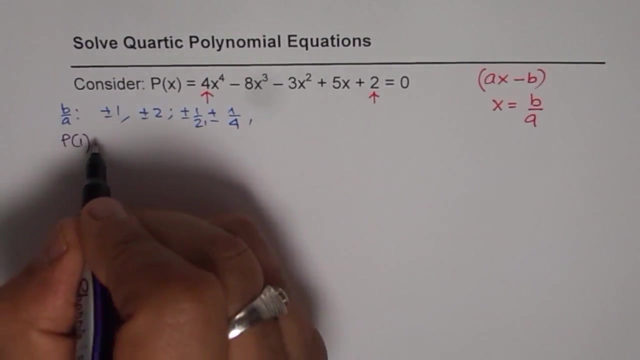 which is already considered. Now let me divide these by 4.. So I get plus minus 1 over 4, and then 2 over 4 is half, which we have already covered. So these are all the values which we could try and get our answer. So let's begin with the first one, which is p of 1.. So let's write the value or the function at 1.. That really means you have to substitute x as 1.. So we get 4, 1 to the power of 4.. Let me 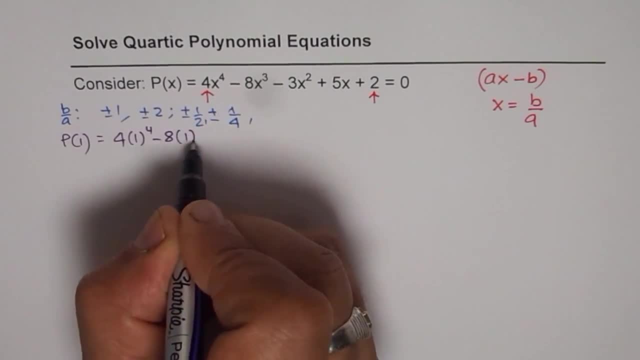 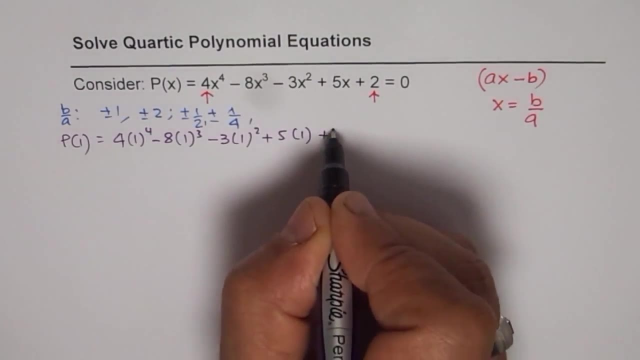 write 1 to the power of 4, minus 8, 1 cube minus 3, 1 square plus 5 times 1 plus 2,. right, You should use a calculator to do all this, but I don't have one today, so I'm just doing rough. 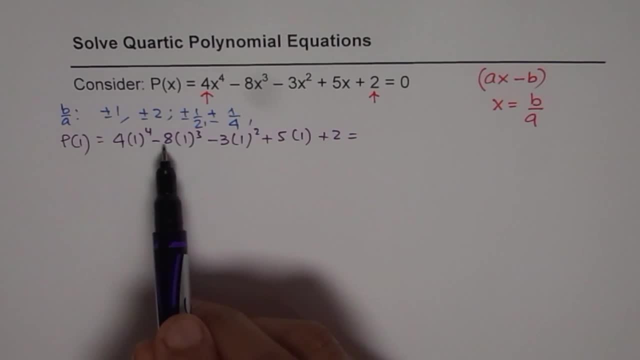 calculations here. So what we get here is 4 minus 8 minus 3 plus 1 plus 2.. Let's add the positive terms: 4 plus 5 is 9,. 9 plus 2 is 11, and negative terms: minus 8 minus 3 is 11,. 11 minus 11 is 0,. 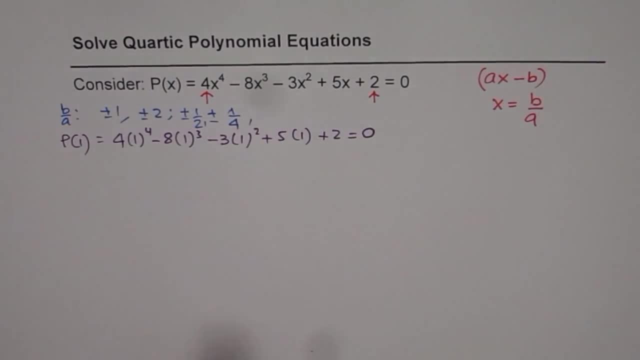 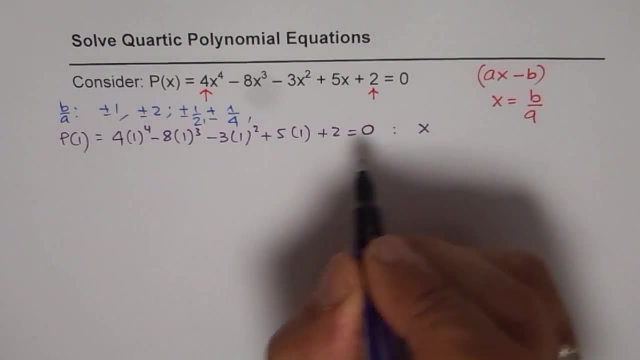 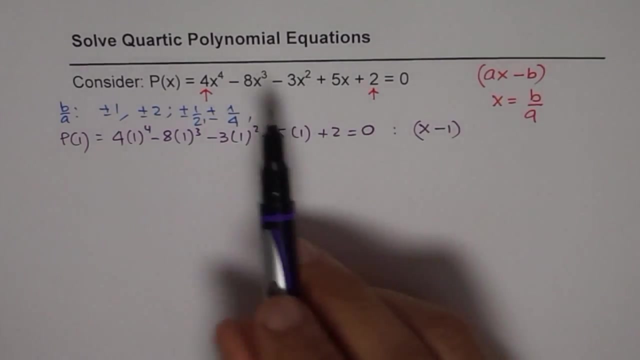 so we are fortunate to get 0 in the very first try, but that's kind of rare. Now, once you get this 0, it really means that the factor is x minus 1, so that is one of the factors of this polynomial. If I substitute 1 here, I'll get a 0, so that is a part of our solution. 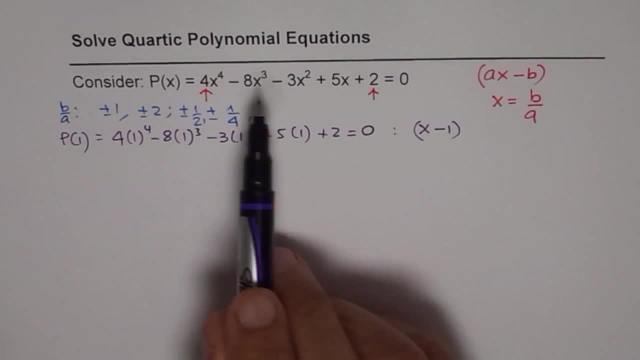 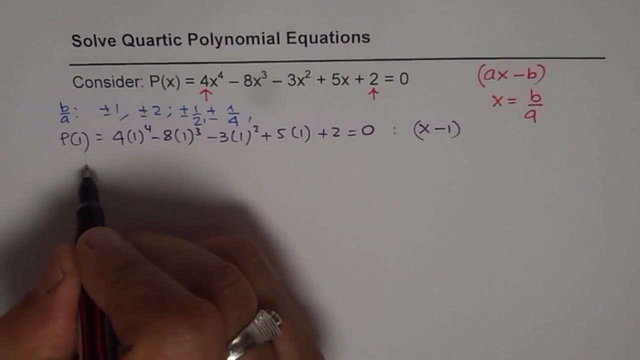 okay, But this also helps us to write this polynomial as a factor of linear factor and a cubic factor. The other one we can get by long division or we can do synthetic division, okay. So let me do synthetic division here, because I'm running out of space most of the time, So we'll do synthetic. 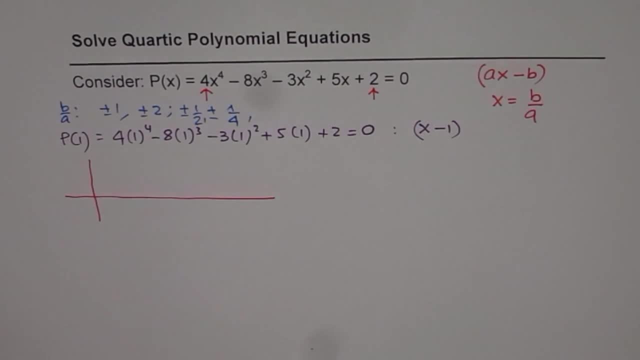 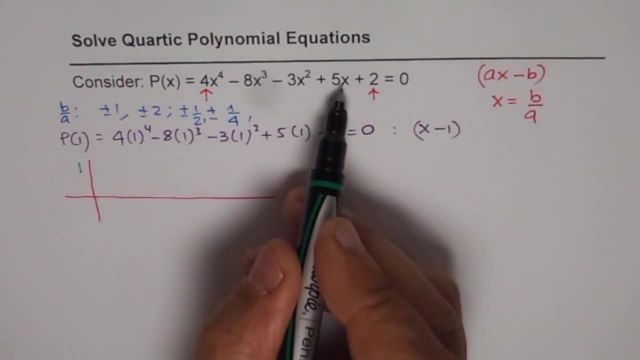 division, and we are expecting remainder to be 0, right, Since x minus 1 is a factor. so we'll divide by 1, and we'll write down all these coefficients. None of the coefficient is missing, so we don't have to introduce a. 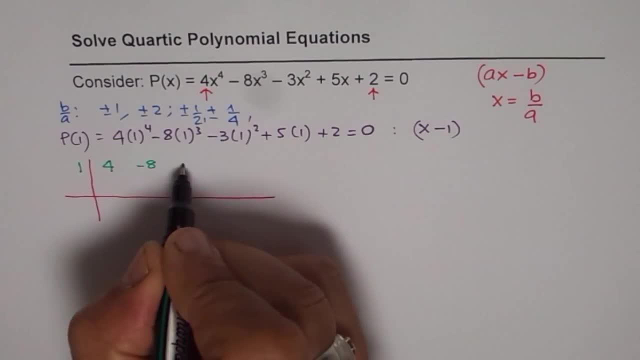 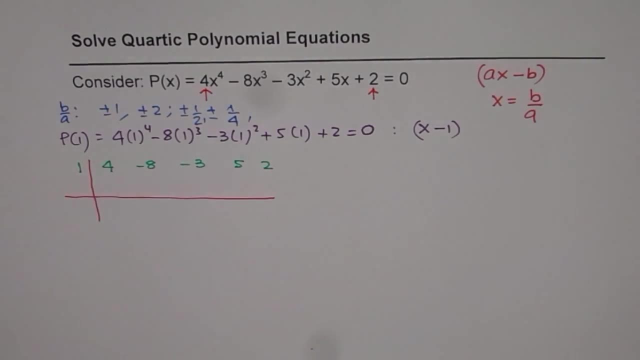 placeholder, right. So we have 4 minus 8 minus 3 plus 5 and 2.. So we bring down 4 here, so we'll use another. it may be good, right? So bring down 4, multiply by 1, you get 4, add them up. 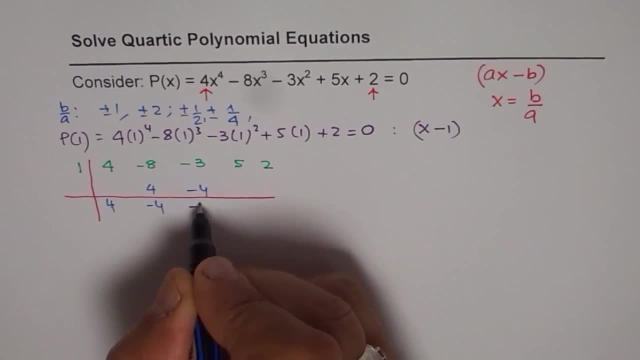 minus 4, multiply minus 4, add them up. minus 7, bring it there minus 7, add them up. you get minus 2 times minus 2, 0. Perfect, So we got a 0, and these are the coefficients of a cubic. 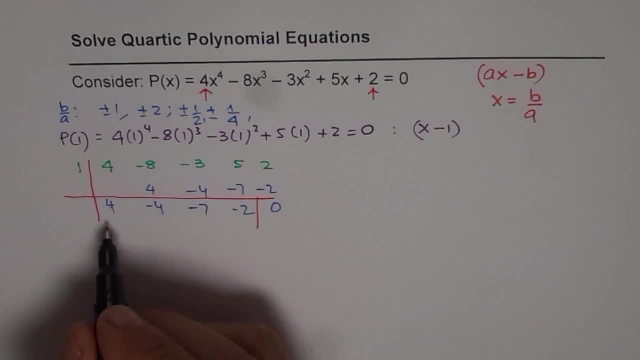 function correct. So these are coefficients of cubic function, which we'll write with the coefficients as 4xq minus 4x squared minus 7x minus 2.. So we got one more factor. now Let me call this another polynomial. So we know. 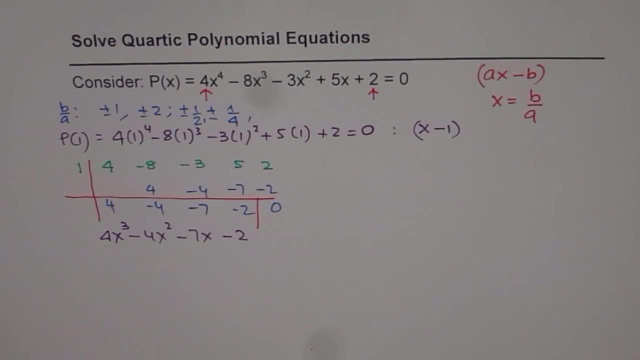 this is x minus 1 times all this. Now the exercise is repeated, We'll again try to figure out what are the possible values which can give us 0 now. So still, you see 2 and 4, kind of similar. 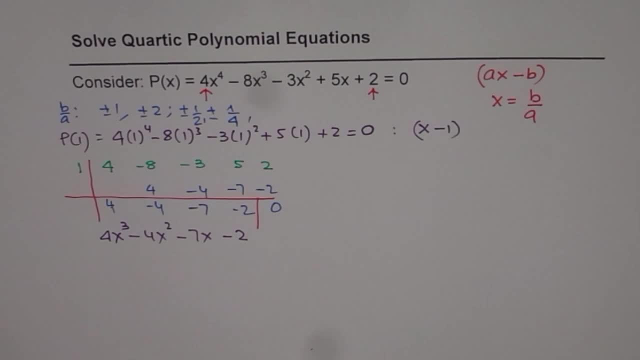 so we're left with the same options. Let's try the next number, okay, So let's try the next number, and we'll try p of 2 now. So we have 4 times 2q, which is 8, minus 4 times 2,. 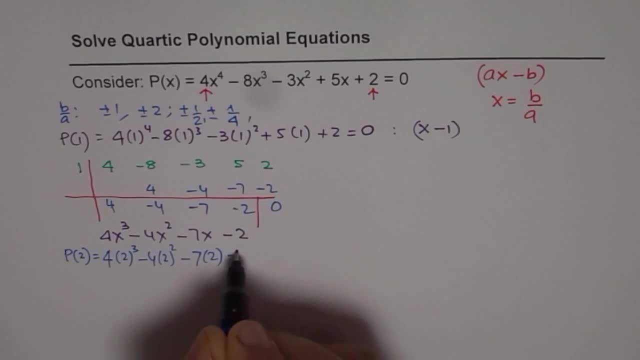 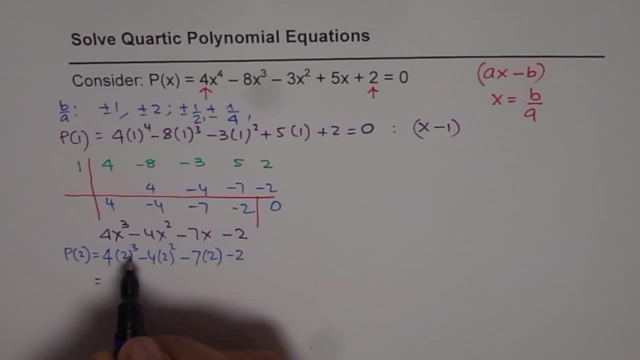 square, which is 4 minus 7 times 2 minus 2, so so we can multiply these numbers and see what do we get. 4 times 8 is 32, right? 2 times 2 is 4, 4 times 4 is 16, and here we have minus 14 and minus 2. 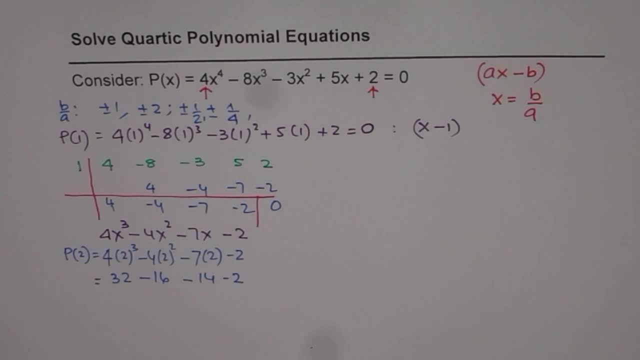 okay, let's add the positive numbers and the negative numbers. okay, so positive numbers is 32. second negative is 16, 14. that means 30 into great job, so that is also 0. you know that there's something good about not working with calculators: you get easy questions to work with. so p of 2 is 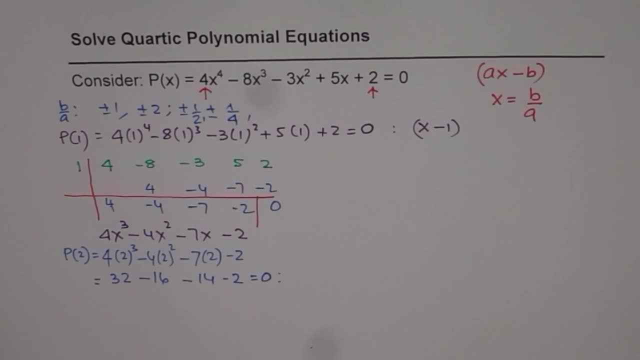 0. that means what that means. we got the second factor, and this one is x minus 2, correct? so if i do synthetic division again, i'll again get a remainder, and then i will know exactly what the quadratic equation is, and we can solve the quadratic equation, since we know a lot of factoring. 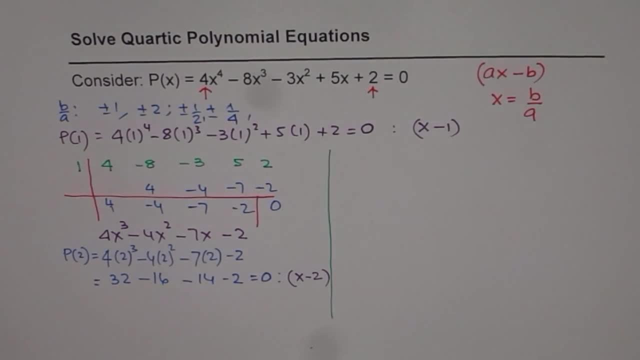 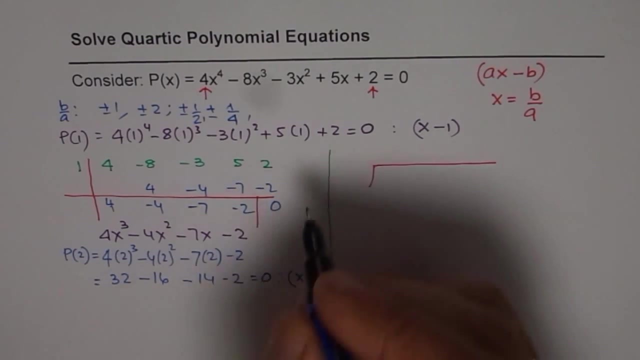 techniques to solve it. this time let me use the long division method to solve. okay, so what we'll do is we'll do long division. this time we have a cubic equation which is here 4x cube, and we are dividing it by 2. perfect, rather the factor x minus 2 this time. yeah, I forgot, we'll do long. 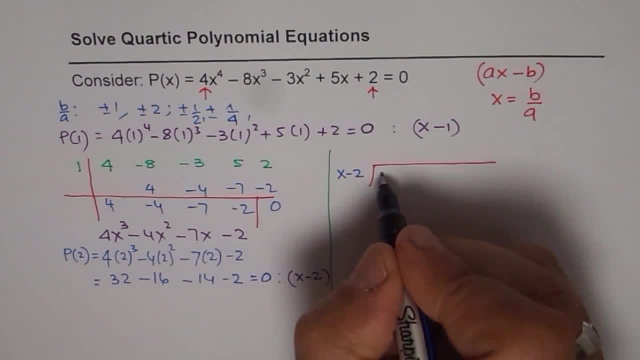 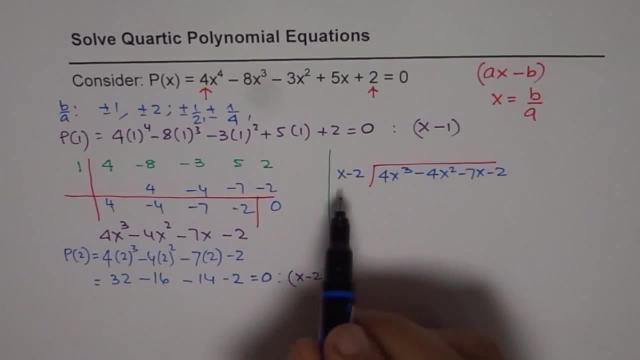 divisions. we'll write x minus 2 here and the equation 4x cube minus 4x square minus 7x minus 2. okay, x minus 2 will take the two terms x 4 and x square. okay, so we get 4x cube. 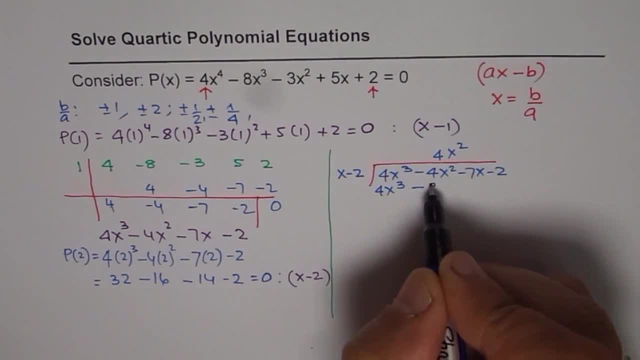 minus 4 times 2 is 8 x square. so when you take away, what do you get? you get plus 4x square. bring down minus 7x. you have to multiply by 4x. now, so plus 4x, okay. so that will give us 4x square minus 8x. okay, and what do we? 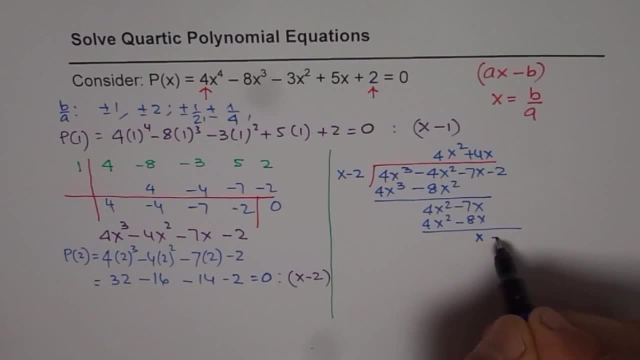 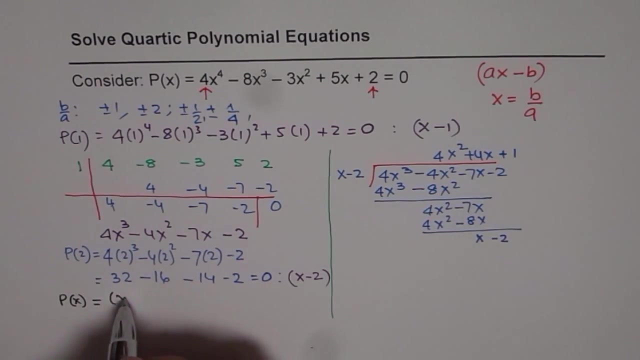 get. when we take away this, we get x minus 2, which goes 1 times so plus 1, perfect. so that is the quadratic factor and we have another factor here. so I think let me summarize by writing the polynomial here. so our polynomial which we are trying to write is: first we got x minus 1. we shouldn't forget about that. 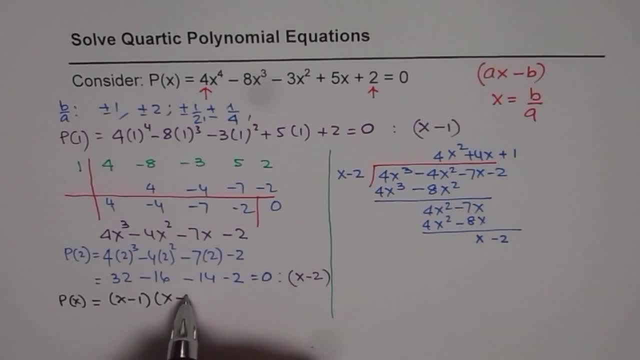 and then we got x minus 2 right there, x minus 2, and when we divide by x minus 2, we got this quadratic function here which is 4x square plus 4x plus 1. so we have all this correct. so at this stage we need to factor the quadratic equation. we can do it by sum and product, we can do it by: 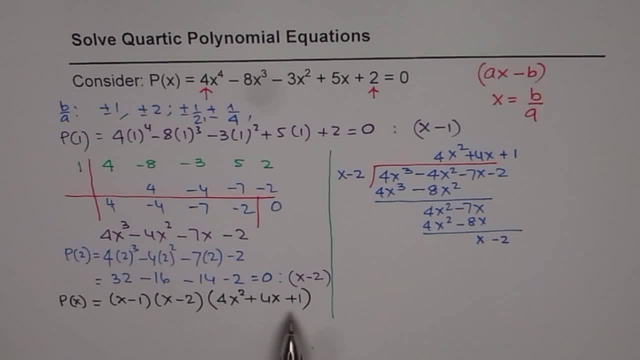 quadratic equation. we have many options. right: sum and product. 4 times 1 is 4 and we are looking for sum of 4 which is 2 times 2. right, so that works. 2 times 2 works, correct, so we can factor this so. 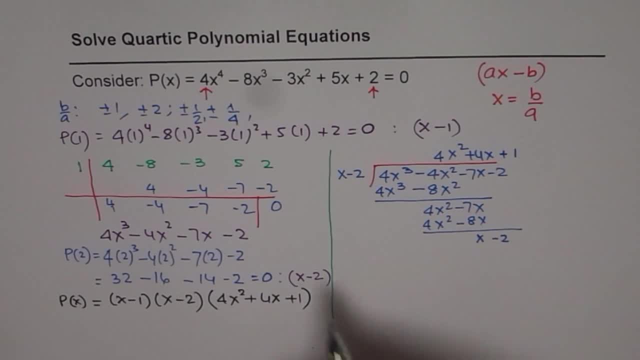 let's do that part. or we can use quadratic formula also, but I think we can use 2 times 2 here, correct? so we will factor 4x square this time. so we have 4x square plus 4x plus 1 and we figure out that the magic numbers are. 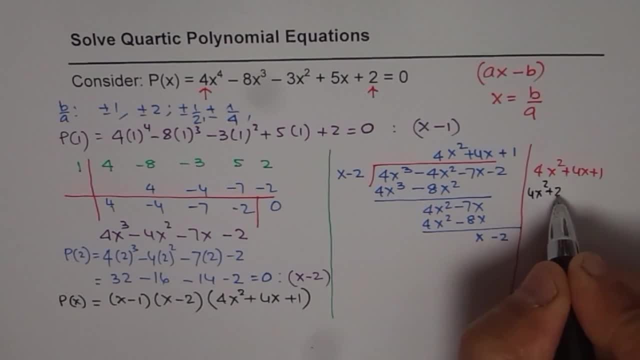 2 and 2, so we have 4x square plus 2x plus 2x plus 1. when we combine these two, 2x is common, so we have 2, 2x plus 1 and we already have plus 2x plus 1 here, so we can take 2x plus 1 and we have 2x plus 1. 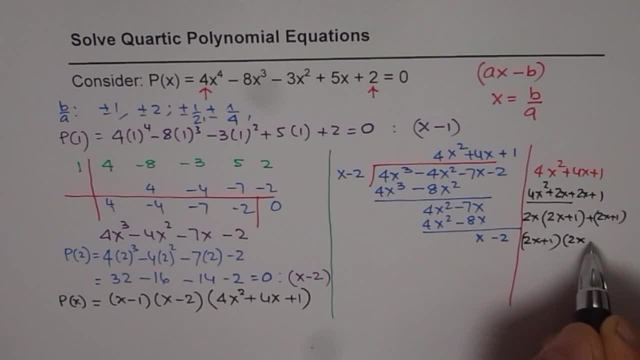 comma right and we are left with 2x plus 1. okay, so it is basically 2x plus 1 whole square, which I could have written here directly, correct: 1 square is 1 and 2x whole square is 4x square, 2 times this. 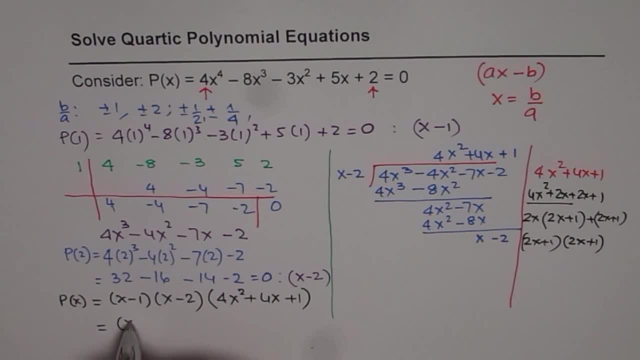 good job. so so we have this as x minus 1 times x minus 2 times 2x plus 1, whole square right. so that is how we can factor our polynomial correct. so well, we have learned different techniques of factoring you could have used. 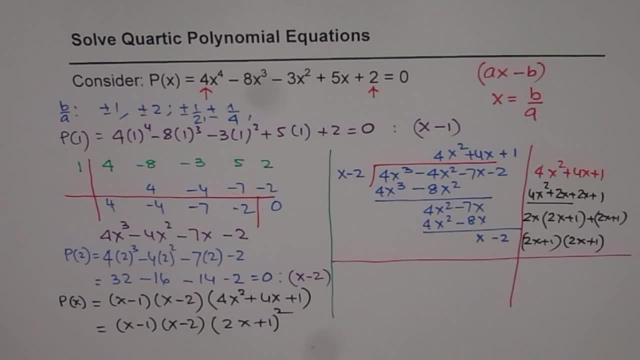 quadratic formula also, or trinomial, you know perfect square. you could have done that also. so basically the question was: solve quadratic polynomial equation. we started with polynomial 4x- 4 degree quartic equation and we need to find solution. what we really found is that this: 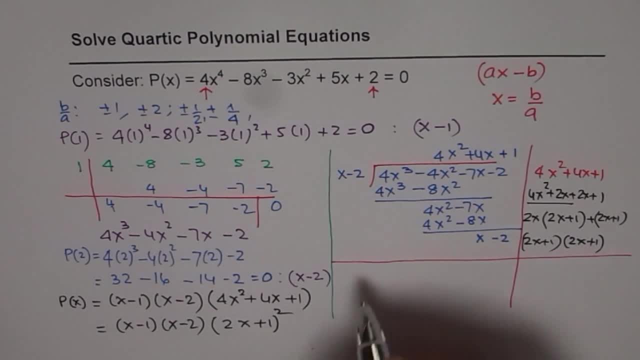 standard equation can be written in factored form, which is x minus 4x, 4x plus 1, and we can write it in a further form. so if you do it in a factored form, it will be x minus 4x, 4x plus 1. 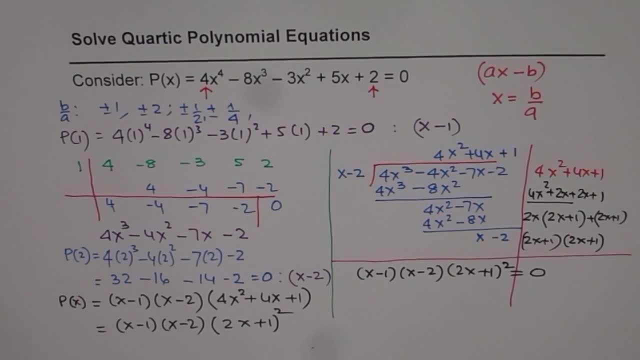 square which is x minus 4x, 4x plus 1, and if you find the solution for the function x minus 1 times x minus 2 times 2x plus 1 whole square and solving means equating it to 0. so now it's a easy part. so 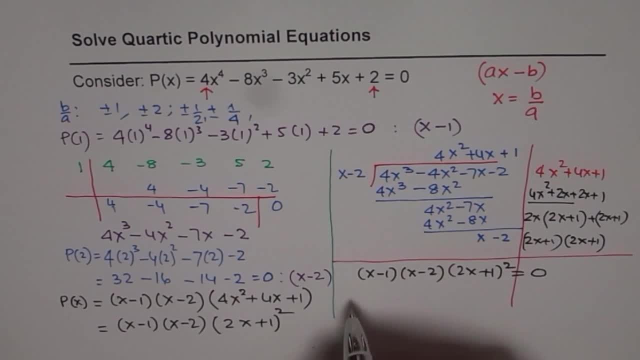 if you are given a factored form, we don't have to do all this, but if not, we have to do all this. to get to this stage, at this stage, we need to find a solution. 1 equals to 0, that means x is equals to 1. right, then we do. x minus 2 equals to 0. that means x. 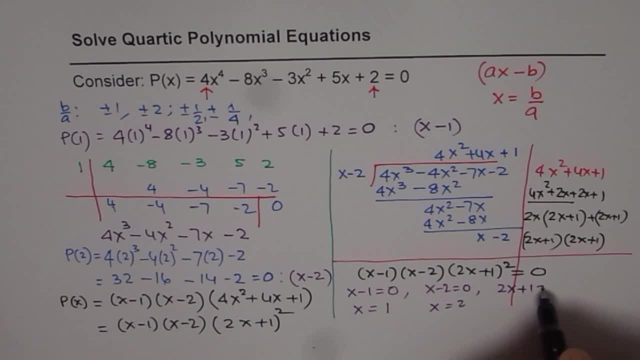 equals to 2. then we do 2x plus 1 equals to 0. that means x equals to minus 1 over 2. so we have three solutions. do you understand? this is a double root. both are at minus half, correct, so we can clearly. 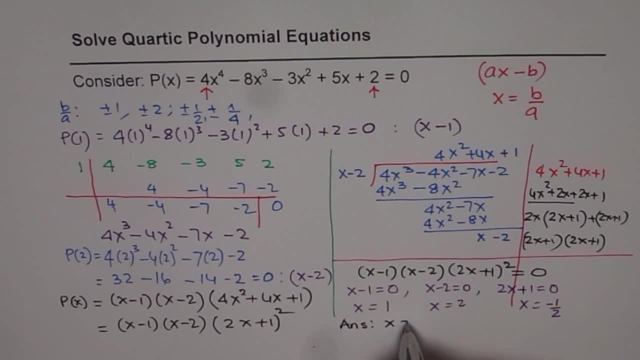 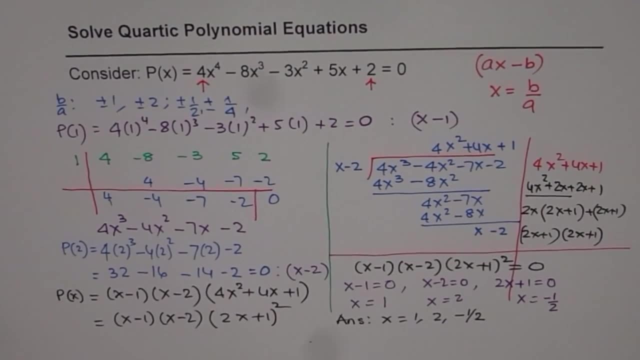 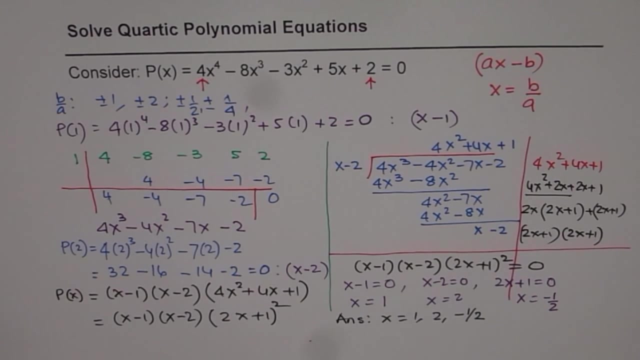 write down our answer now. our answer is: x is equals to 1, 2 and minus half. okay, so i hope with this you understand how to solve a polynomial equation. i have purposely taken a very simple example. the idea is not to impress you, but to tell you a method of doing things right at times. 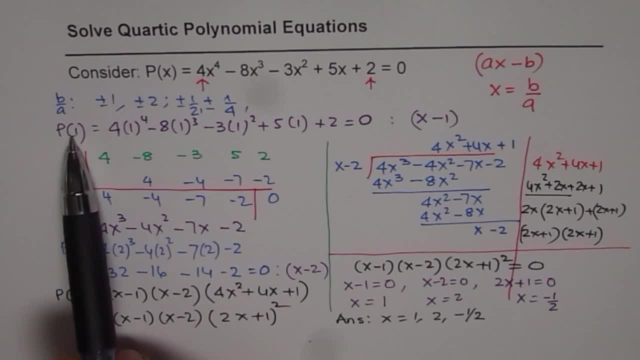 the numbers can be very complicated. you may have to try a couple of times before getting the first zero itself right. but don't forget, get disheartened, keep trying. so that is the whole I can tell about it. but follow the method, you will definitely get the answer quickly. thank you and all the 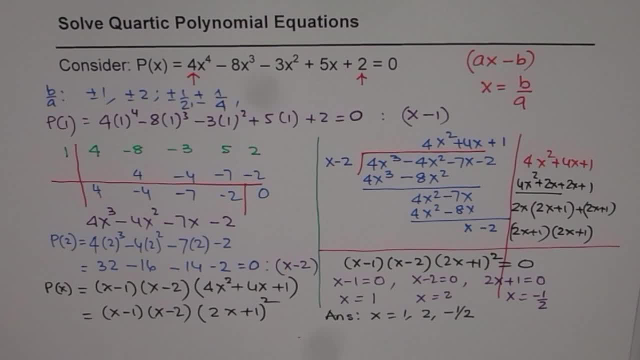 best. don't forget to subscribe to my videos. I'm Anil Kumar and thank you once again.